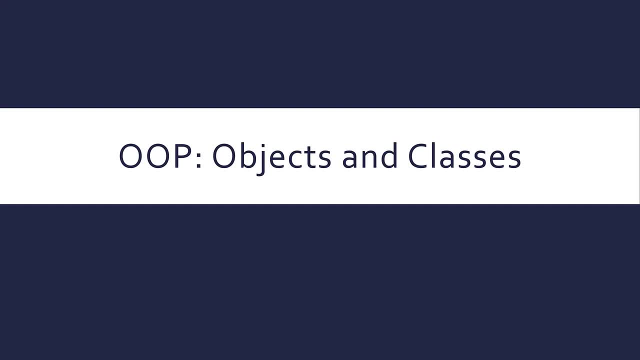 Hello, this is the first in a few videos on the object oriented paradigm. I'm going to really try and build this up bit by bit, because there's lots to cover, way more than procedural paradigms, because there are lots of terms to learn and lots of just ideas to get across. Now I'm going to leave why until right at the end, like why are we doing this? Why is this a paradigm? Because I think you can't fully appreciate it until you've understood a lot of the concepts involved. Now what I would say is, to be honest, not this video, but other videos will include terms which vary quite a lot per language. 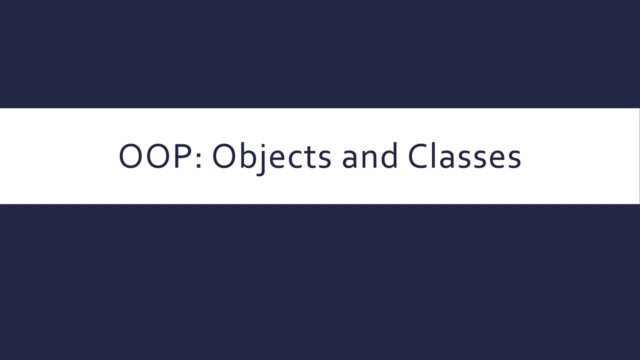 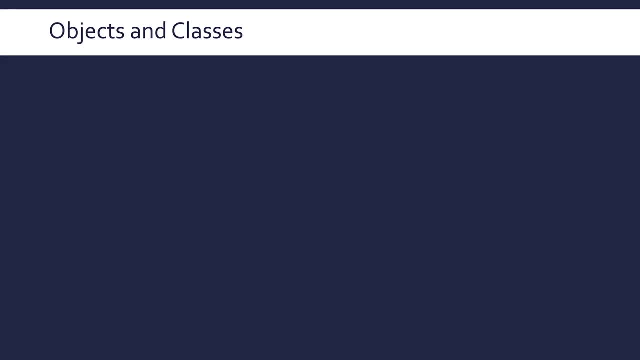 Frustratingly, to an extent, different languages implement these ideas in different ways. I'm going to try and take this from a more theoretical perspective. Just make sure, if you are doing a practical exam, you've got knowledge in your particular language. 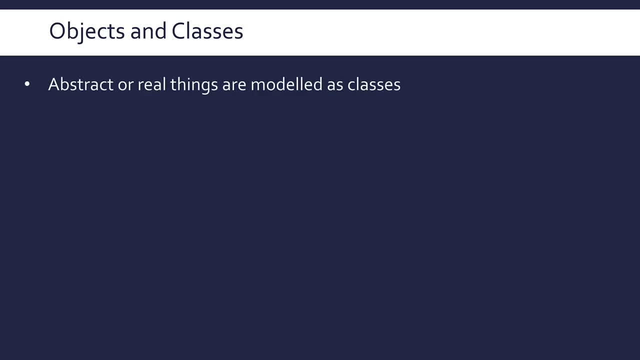 Now, what is applicable to every language are just the high level concepts of objects and classes within object oriented programming. The first thing you do when you're programming in an object oriented way is you try and model things As a class. Now, what you're modeling can be both abstract or real. 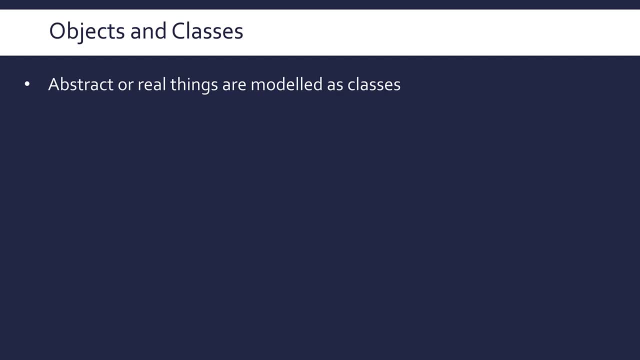 So: abstract meaning, it's detached from reality. Real meaning, it's an actual, real life thing. So to give an example of a real life thing, let's say we are trying to model a dog, So we've got a program which is making use of a dog. Whether you do this for real I'm not sure, but it's, I think, fine for a first example. 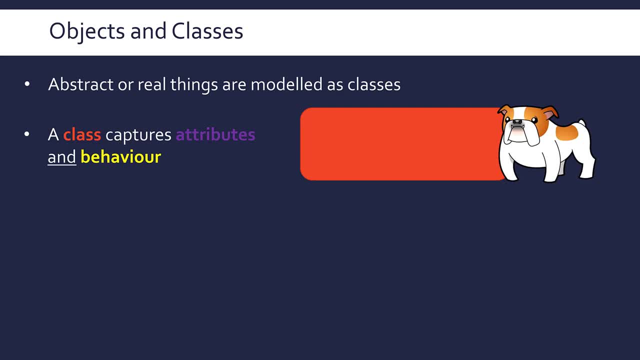 So a class is this entity in programming, And the purpose of a class is to capture two things. It's to capture the attributes of this- either abstract or real thing- and its behaviour. So we're separating these things into their attributes and their behaviour. 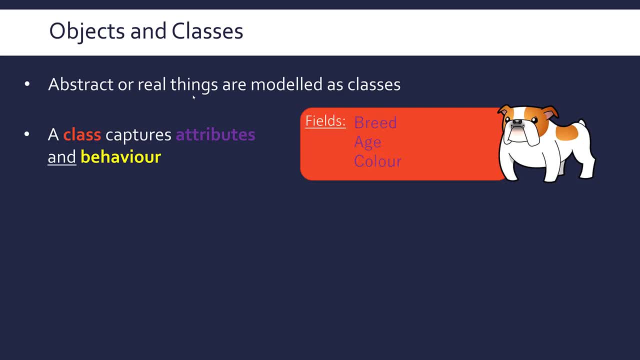 So attributes are just kind of cold boring properties of the thing. So for a dog, things like breed, age, colour, height, weight, the name of the owner, etc. etc. It's just a bit of data about the dog. 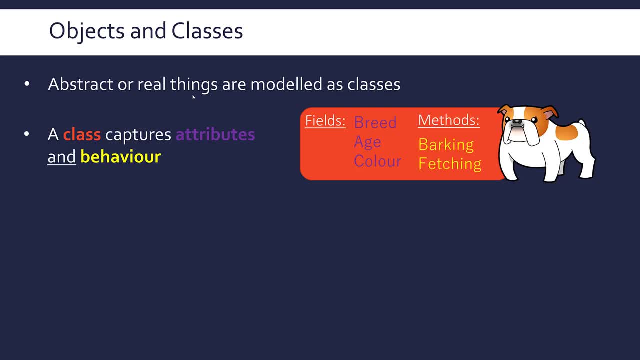 Whereas behaviours are things which our thing does. So for a dog, things like barking, fetching, running, eating, drinking, sleeping, Things which it does not, things about it. Now, I've put fields and methods in my little class here, because often attributes and behaviour are sort of our theoretical terms. 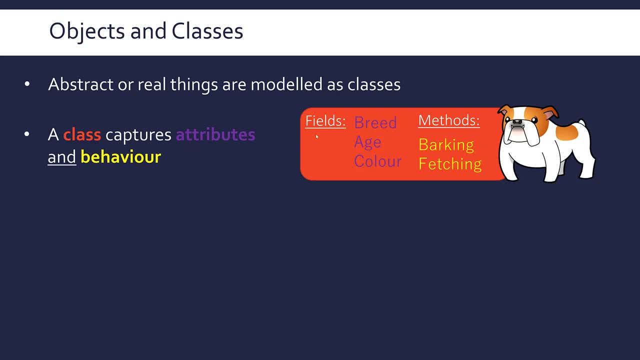 When we go to implement these in code, we then call attributes, fields and behaviours methods, But I'll come back to that a bit later. So a class can think of as just being like a box which contains details of the fields and the methods. 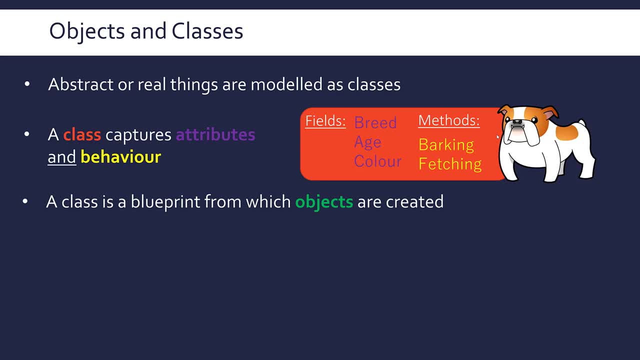 Now, really, a class itself is a blueprint. So a class on its own is not very useful. All it does is provide a general template for us to create objects. So a dog class is just for a generic dog. It should apply to ideally every dog. 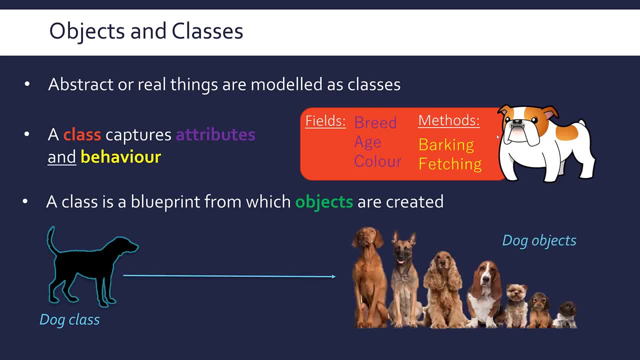 But what we can do is we can create objects Which are specific instances of a dog. So the point of a class is to represent all objects of that specific type, In this case dogs, Whereas an object is an actual, concrete example of the class. 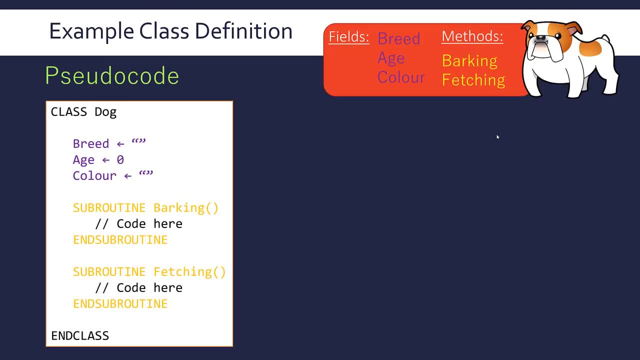 Here's how we might actually define this in code, or at least pseudocode. So it will vary depending on the language. We've got the two sections of our class. The class is just a definition. Again, when it is a class, It's just a template. 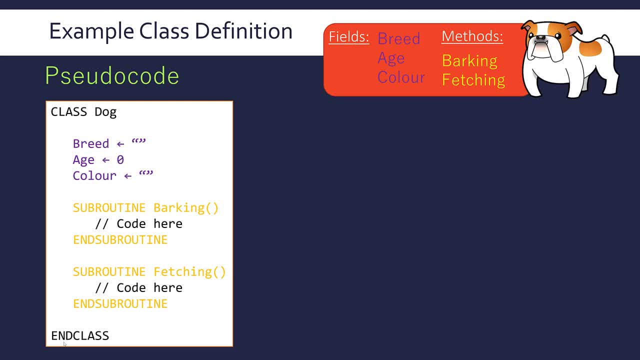 It's not for an actual specific dog yet It will be once we make an object based on this class. We've got the two areas, We've got our attributes usually at the top And we've got our behaviours usually at the bottom. 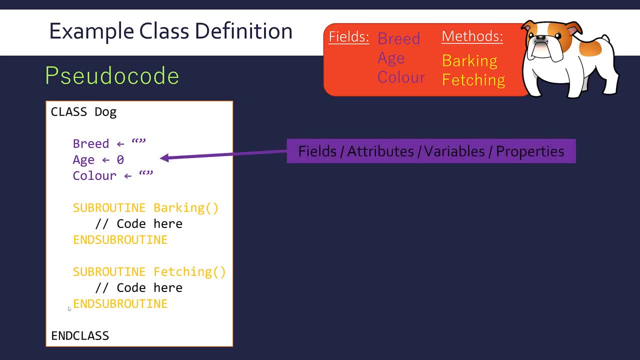 Now what can be confusing if you're starting to learn object-oriented programming is terminology varies a lot, So your attributes can be called attributes, But also can be called fields. Can just be called variables, because that's what they are, And in some even looser senses they can just be called properties. 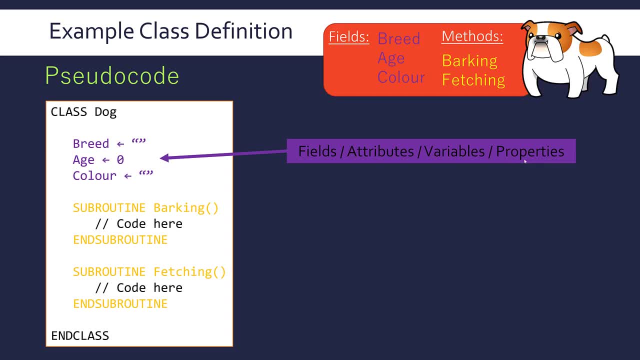 Although in a language like Java that doesn't tend to apply in that way, So it varies a little bit. I tend to say fields and attributes. There are different types of variables within object-oriented programming, which I'll come back to in a future video. 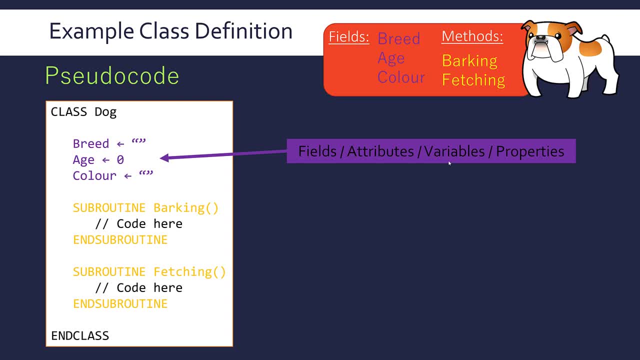 So I wouldn't worry too much about the terms you're using And don't get too put off if you hear slightly different words for these concepts For our behaviours. rarely will they be called behaviours In an actual code context. usually they're called methods. 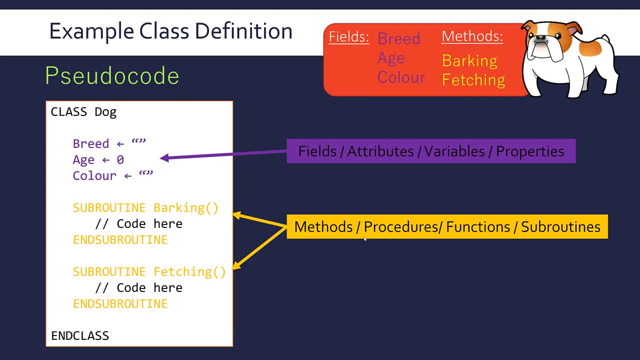 So a method is a subroutine which is within a class. So methods really only apply in object-oriented programming. They don't really apply in procedural programming. But the actual methods can be either a procedure or a function. So in procedural programming we tend to teach it that functions return a value, whereas procedures do not. 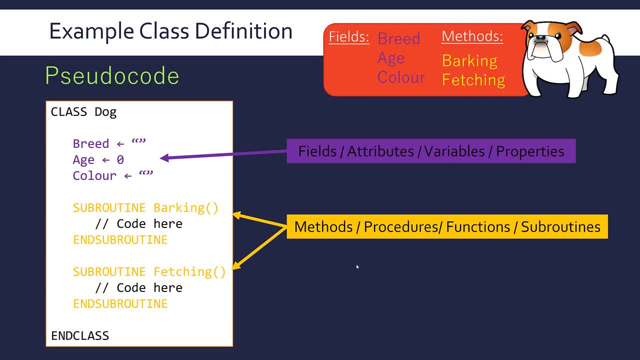 Well, either one. So a method inside a class is called a method in this context, But you may still hear them called procedures and functions. A method can return a value, It cannot, And the general word for what these are? just blocks of code, are subroutines. 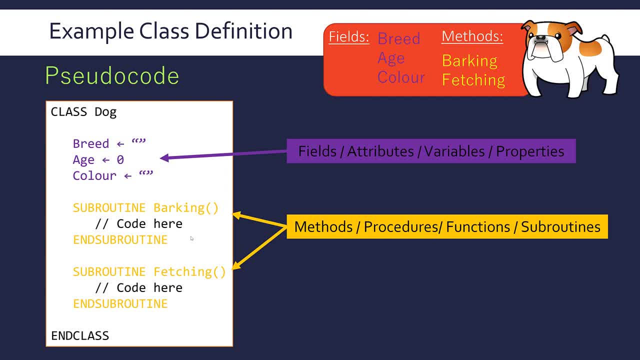 So we represent the behaviours as subroutines And you would define them pretty much exactly the same as you would normally, just inside your class. Now, because this is a template, I've just set my fields to be just initial values. But ultimately, if I make a template, 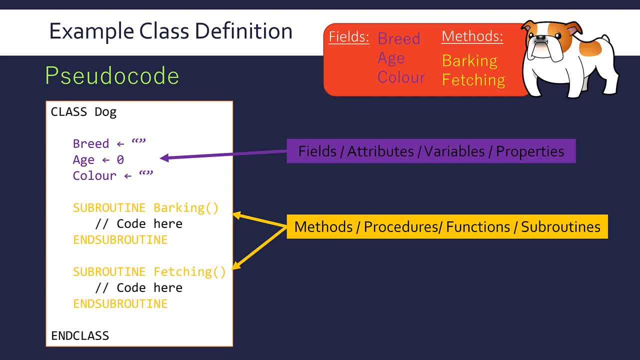 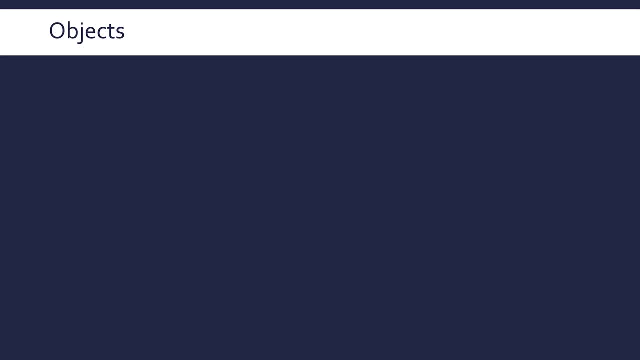 if I make an object, which I'll focus on more in the next video, I'll give specific values to these fields. So just a little bit more about objects before I talk about that in the next video. Each instance of a class which is an object can have, and will most likely have, different attribute values from each other. 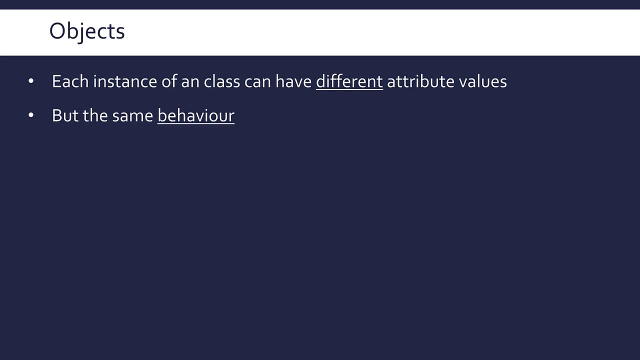 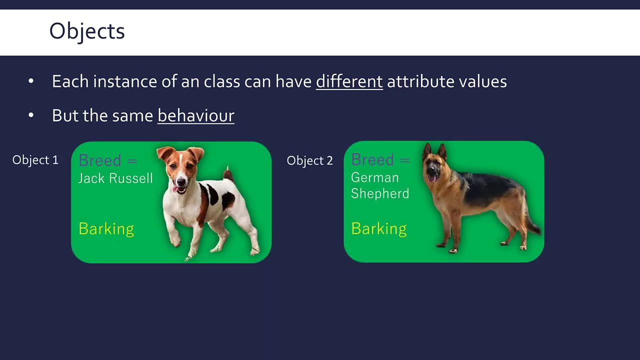 But the behaviour will be common across every object. you have Meaning that those subroutines apply to every object, even if the actual field values vary a little bit. So this tracks from real life, right? Dogs are very different, The different breeds of dogs are very different. 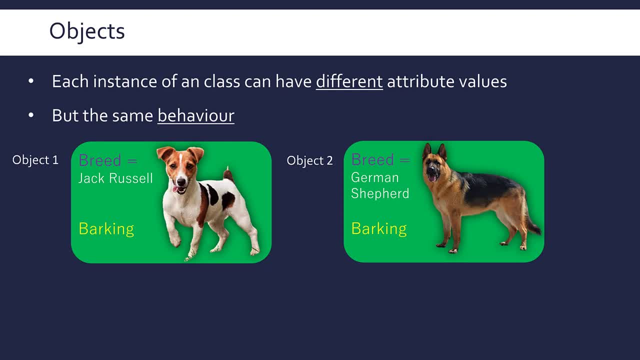 But they are still dogs, So they've still got the same common attributes like breed, But the actual values are different And it has a different effect on the behaviours. So while a Jack Russell and a German Shepherd both bark, clearly, they bark in a very different way.